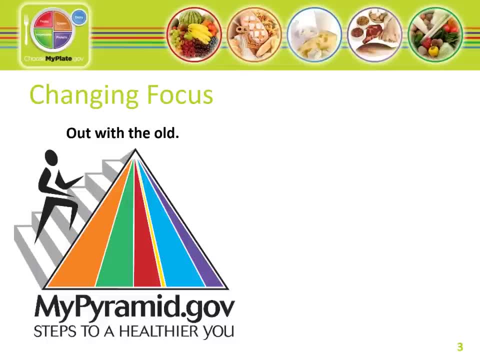 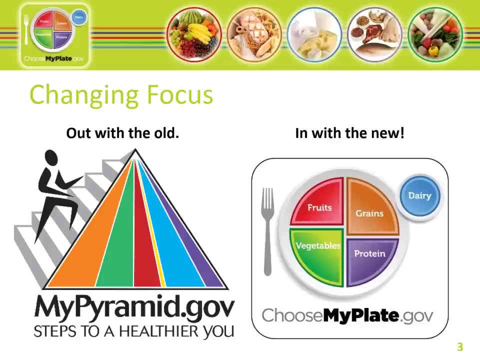 and understand What did the stripes mean And why were some stripes whiter than others? The MyPlate icon is easier to follow. With MyPlate you can visualize that you should make half your plate fruits and vegetables, a quarter grains, a quarter protein and dairy. The 10 tips to a great plate are: 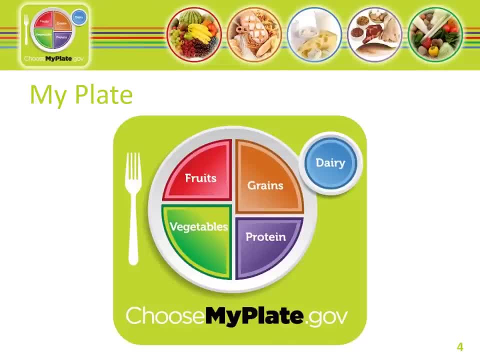 balanced calories. enjoy your food, but eat less. avoid oversized portions. eat fruits, vegetables and whole grains. often make half your plate fruits and vegetables. switch to fat-free or low-fat milk. make half your grains whole grains. eat less solid fats, sugar and salt. compare sodium in food and drink water instead of. 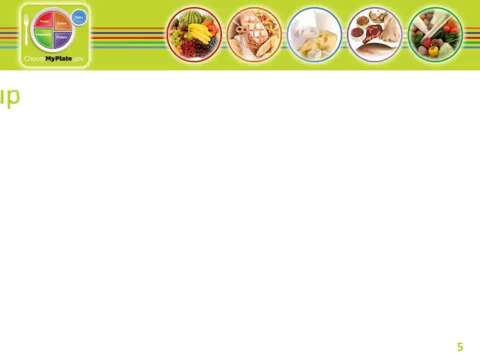 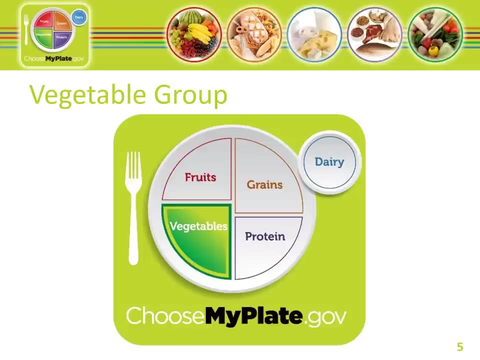 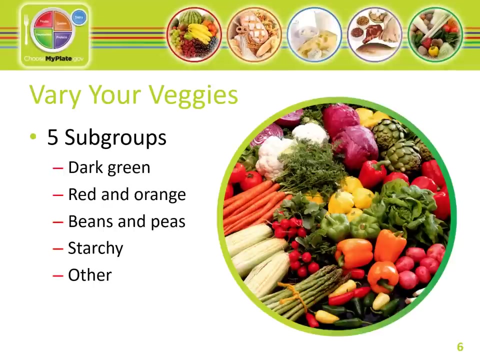 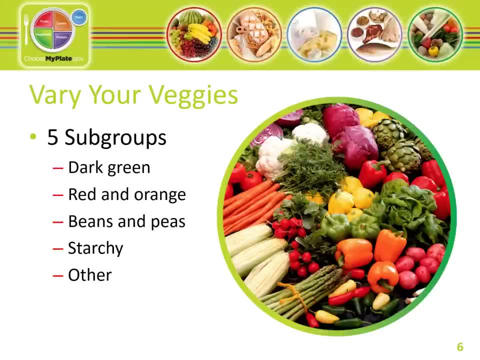 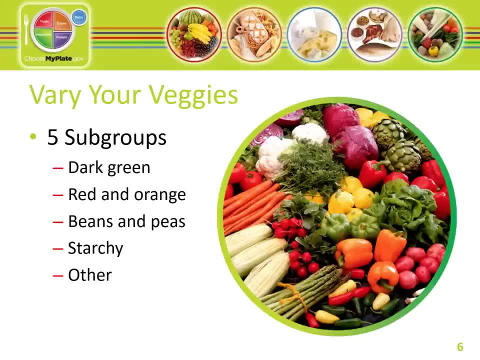 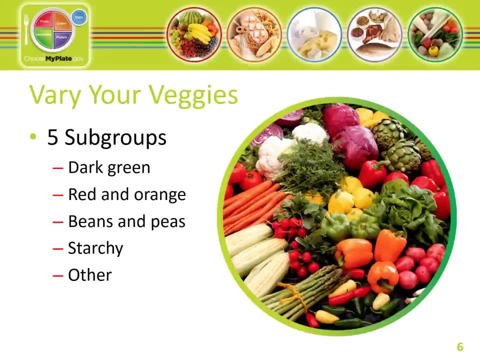 spinach and brussels sprouts. Some commonly eaten vegetables in each subgroup are dark green vegetables such as broccoli, spinach and brussels sprouts. Some commonly eaten vegetables in each subgroup are dark green vegetables such as broccoli, spinach and brussels sprouts. 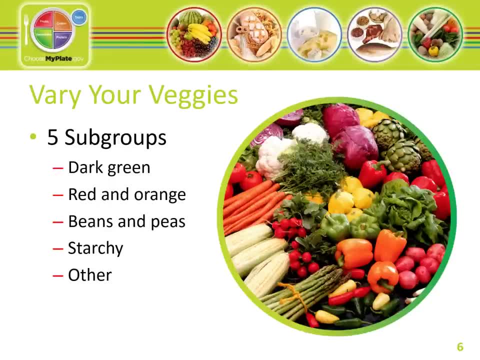 spinach and Brussels sprouts. Red and orange vegetables include carrots, pumpkin, red peppers, sweet potatoes and tomatoes. Beans and peas include black beans, kidney beans, lentils, soybeans and split peas. Starchy vegetables can include corn, green peas, plantains and potatoes. Other vegetables, such as 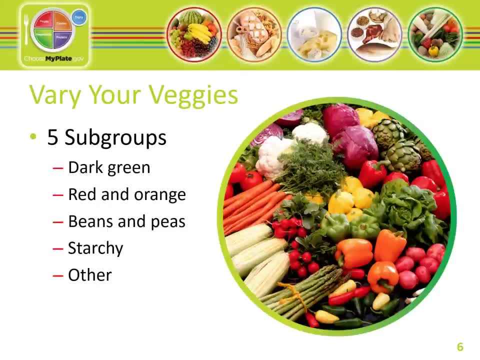 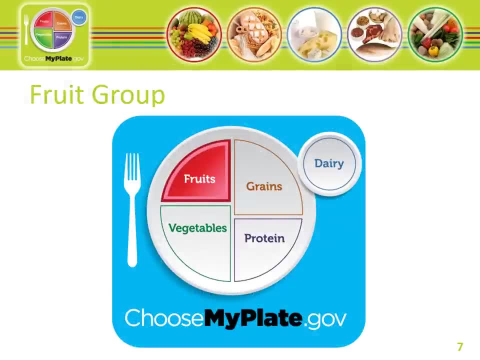 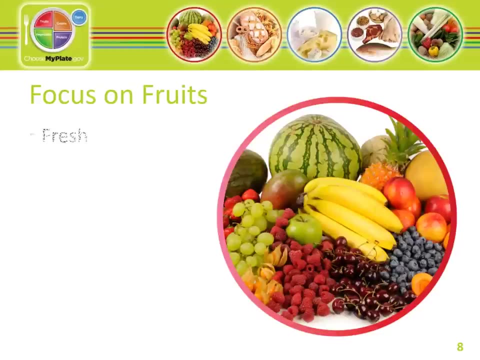 artichokes, asparagus, avocado, eggplant, onions and cucumbers. Next is the fruit group. Here, too, color is important. The more colors you eat, the better. Make half your plate fruits and vegetables. Any fruit or 100% fruit juice counts as part. 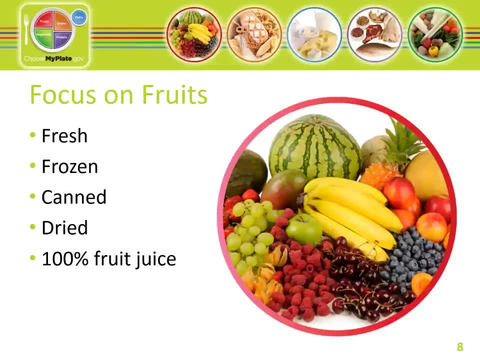 of the fruit group. Fruits may be fresh, canned, frozen or dried. It may be whole, cut up or pureed. Some commonly eaten fruits are apples, bananas, cherries, peaches and pears. The berry group includes strawberries. 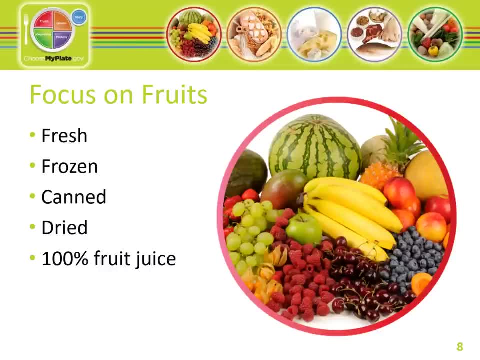 blueberries and raspberries. Melons include cantaloupe, honeydew and watermelon. You may find mixed fruits in a fruit salad or fruit cocktail. 100% fruit juice can be found in orange, apple, grape and grapefruit juice. 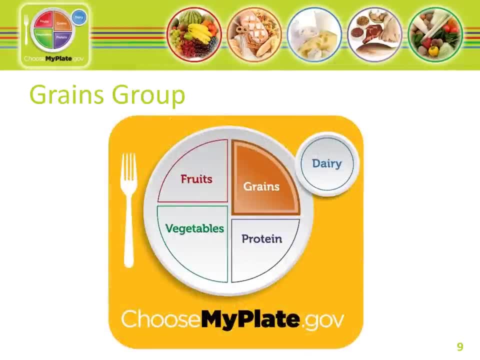 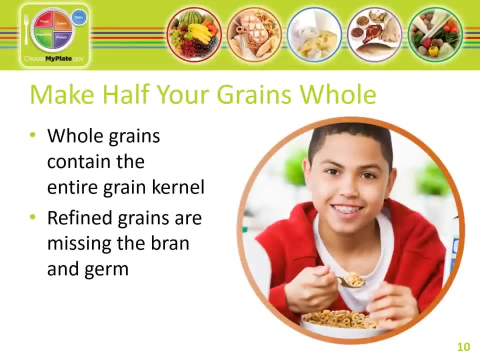 Wholesale food products such as hand mixer, hibiscus and breakfast minus two for one. We're not looking at the ingredients that are the most common here in Canada. Just what you need is a food that has the most کب pää to the whole that matter. Here is the recipe. 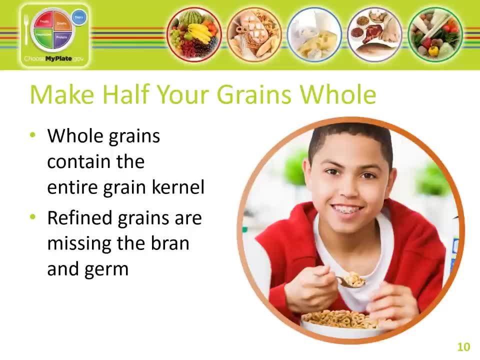 refined grains. 100% whole grains contain the entire grain kernel. They are the most nutritious grain choices and add essential fiber to our diet. My plate recommends that 50% of our grains be whole grain. Examples include whole wheat flour, whole wheat pasta, rolled oats, quinoa, brown rice and popcorn Refined. 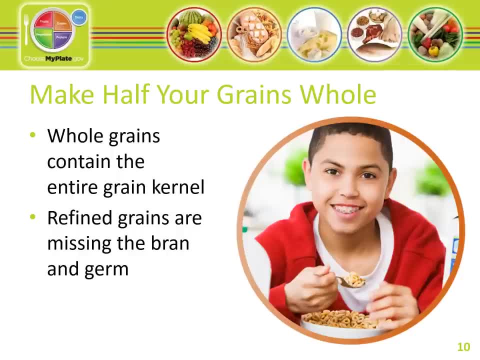 grains have been milled. This is done to give grains a finer texture and improve their shelf life. However, it also removes lots of nutrients such as fiber, iron and many B vitamins. Some examples of refined grain products are white flour breads. 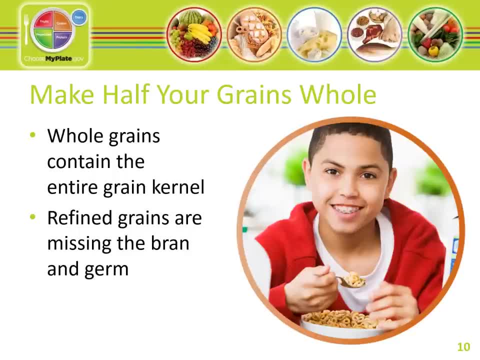 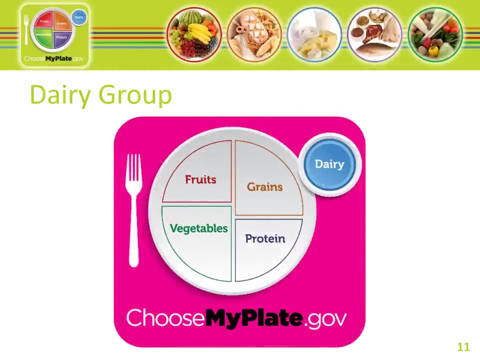 white rice cookies, saltine crackers, cake and pie. The best way to know if you are eating a whole grain is to check the ingredient list on the package. The first ingredient should say whole grain or whole wheat. Dairy foods can provide vitamin D, potassium and phosphorus, in addition to calcium. 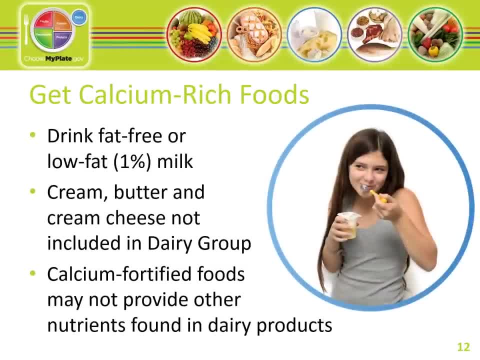 Switch to fat-free or low-fat 1% milk. Foods included in the dairy group are milk, yogurt and cheese. All milk and many foods made from milk are considered part of this food group. Dairy group choices should be Fat-free or Low-fat. Foods from this group provide vitamin D, potassium and phosphorus. 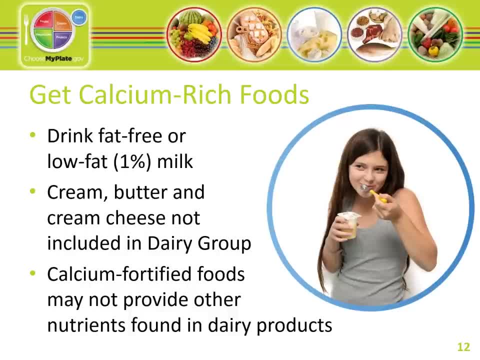 However, foods made from milk which have little to no calcium, such as cream, cheese, cream and butter, are not included. If you choose milk that is not fat free or cheese that is not low fat, the fat in the product count towards the Empty Calories category. If sweetened table- 거죠 or plain 않은. 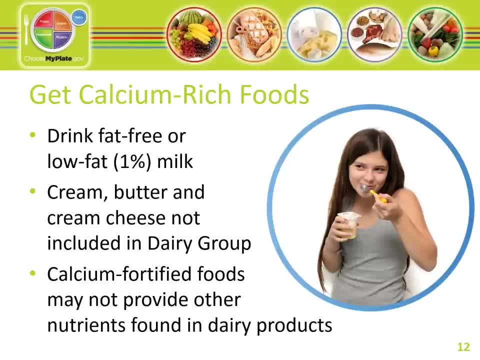 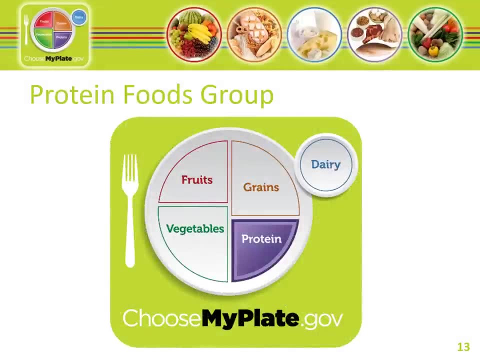 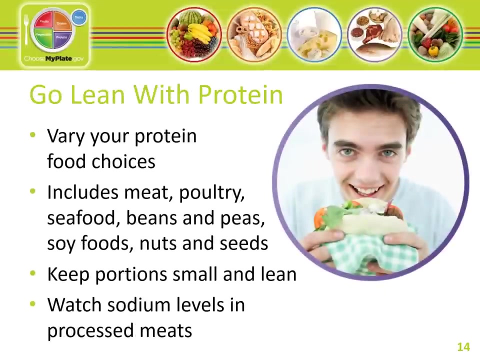 If sweetened products are chosen, the added sugars also count towards your empty calories category. If you are lactose intolerant, you may still find lactose-free or lower lactose products available. Next is the protein group. Select a variety of protein foods to get as many health benefits as possible. 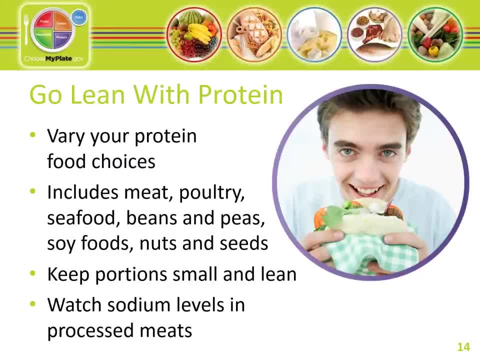 Vegetarian options in the protein foods group include beans and peas, processed soy products and nuts and seeds. When choosing protein foods, keep your portions small and lean. Portion sizes should be 3 or 4 ounces cooked, which is about the size of the palm of your. 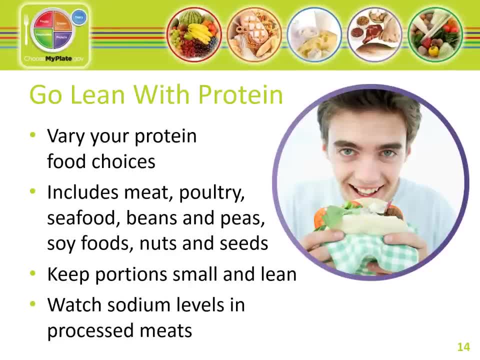 hand, All foods made from meat- chicken, turkey seafood or fish, beans and peas, eggs, processed soy products, nuts and seeds are considered part of the protein foods group. Processed meats such as ham, sausage, hot dogs and deli meats can be considered protein. 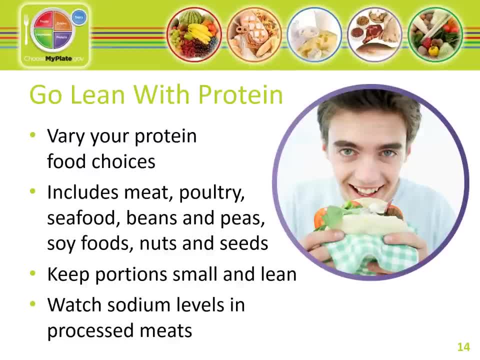 foods. If you are a vegan, you can have a lot of added sodium. Check the nutrition facts label on packages to help cut back. Select fish that is rich in omega-3 fatty acids. The omega-3 fats are good for your skin, your blood, your muscles and your brain. 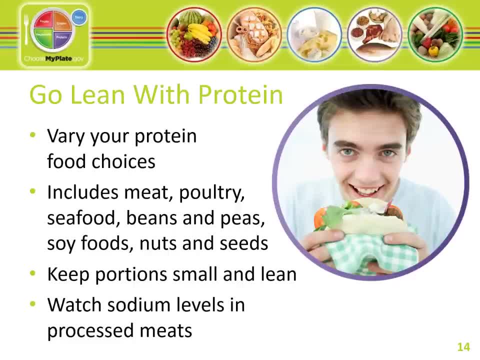 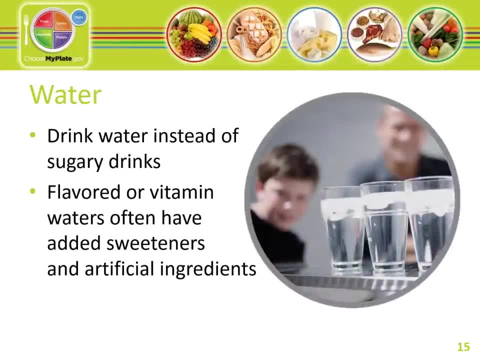 Fish with omega-3s include salmon, tuna, pacific oysters and mackerel. When you are thirsty, water is an excellent choice to drink. It provides the fluid your body needs to keep you cool. 3. Don't dispose of waste and help circulate nutrients throughout your body. 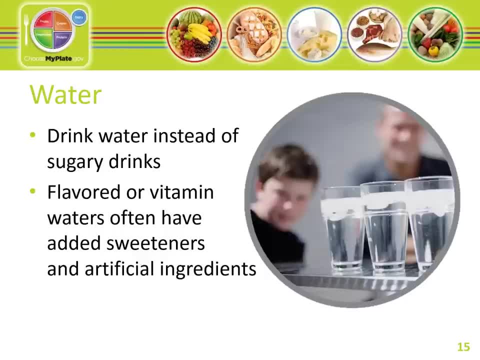 The general tip is to drink 8-ounce servings of water each day. Be sure to have water available when outdoors or doing other physical activity. Not drinking enough water can lead to overheating and dehydration. Flavored waters or vitamin waters in sports drinks usually have added sweeteners and artificial. 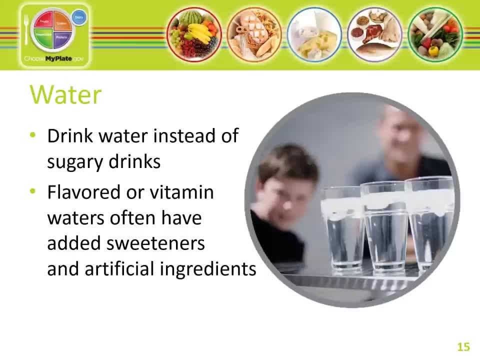 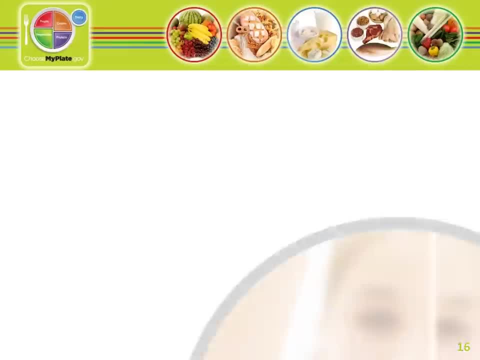 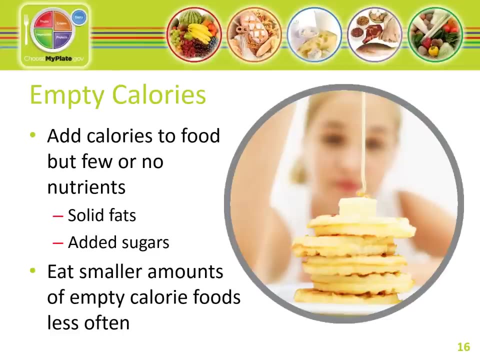 ingredients. The added sweeteners in these drinks add to your diet. 3. Add calories. Be sure to read the nutrition facts label and ingredients on these beverages. Many of the foods and beverages Americans eat and drink contain empty calories. Empty calories are calories from solid fats and or added sugars. 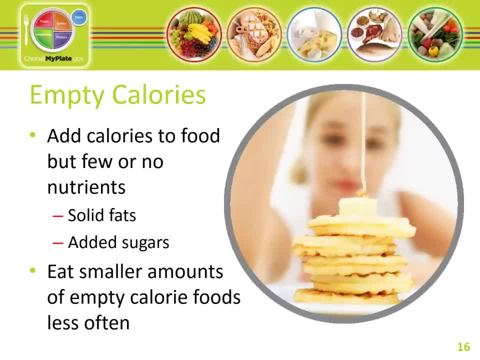 Foods containing high amounts of solid fats and added sugars add calories to the food, but few or no nutrients. 3. Solid fats are fats that are solid at room temperature, like butter, beef fat and shortening. Added sugars are sugars and syrups that are added when foods or beverages are processed. 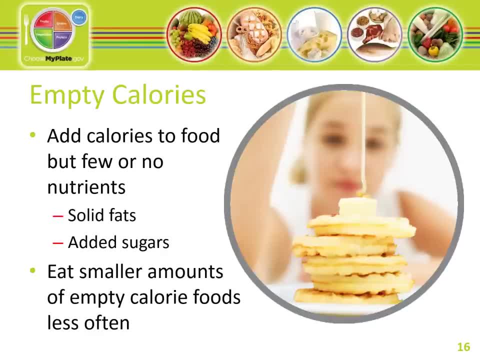 and prepared. The foods and beverages that provide the most empty calories for Americans include cakes, cookies, pastries and donuts, sodas, energy drinks, sport drinks and fruit drinks, cheese, pizza chips and french fries, ice cream, sausages, hot dogs, bacon and ribs. 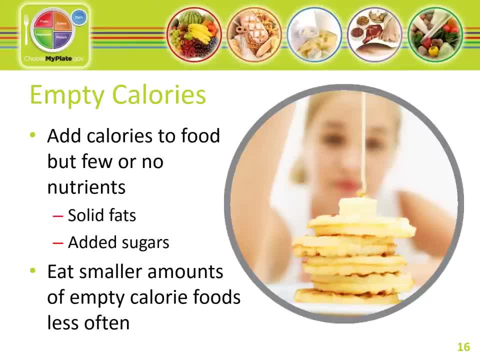 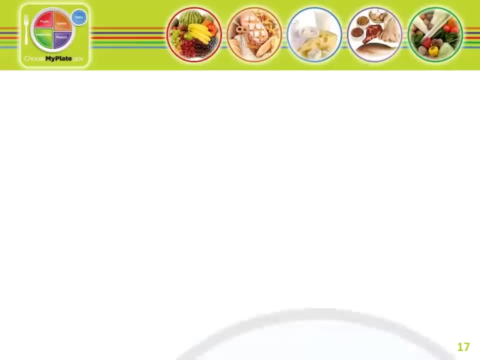 Many of these products contain both solid fat and added sugars. You can find ways to cut the fat and added sugars by looking for lower fat versions of these products. You can choose water, milk or sugar-free beverages instead of drinks with sugar. We all need to be active every day. 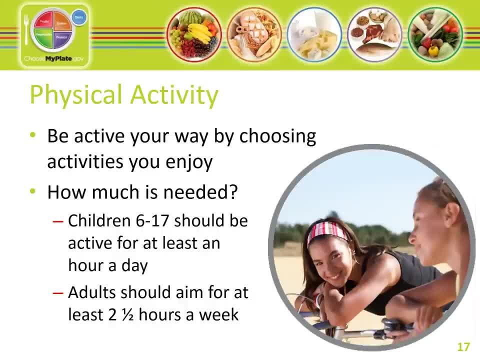 Eating right and being physically active are the keys to a healthy lifestyle. It affects your mood, your brain power and your body's ability to metabolize or burn calories. Physical activity is using energy to move your body: Walking, gardening, biking, climbing the stairs, playing soccer or dancing the night away. 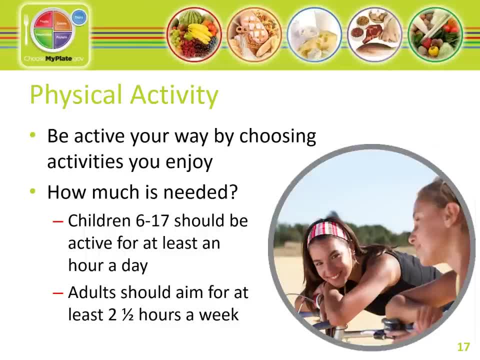 are all good examples of being active. MyPlate defines three activity levels based on the amount of time you spend on your food. 1. The amount of time a person spends being physically active during the day. These are sedentary, moderately active and active. 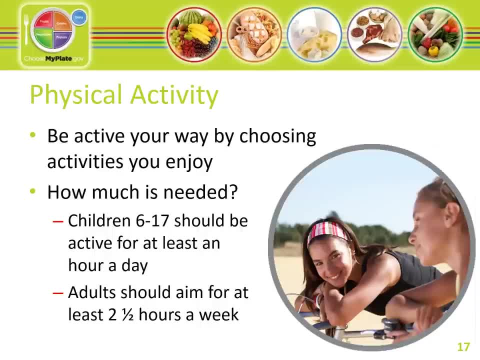 A sedentary activity is when a person gets 30 minutes or less of physical activity in a day. Moderately active is 30 to 60 minutes of physical activity. An active person has more than 60 minutes of physical activity in a day. 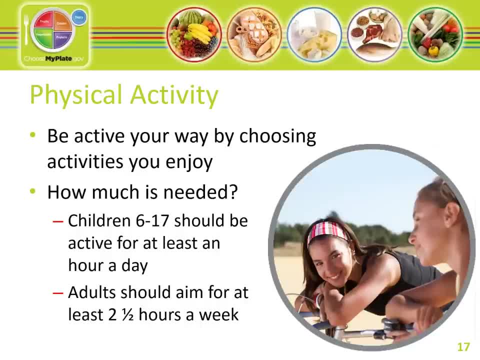 For health benefits, physical activity should be moderate to moderate 2.. The best way to incorporate physical activity into your day is to pick activities that you like and start by doing what you can, at least 10 minutes at a time. Every bit adds up and the health benefits increase as you spend more time being active. 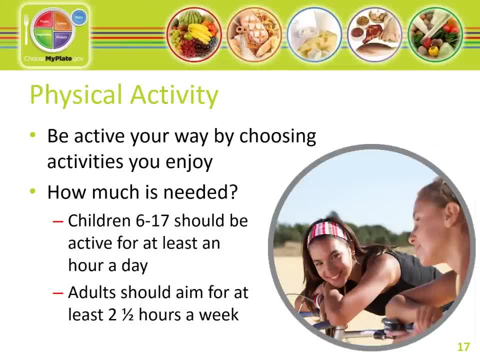 Youth should be active for at least 1 hour every day At a minimum. adults and older adults should aim for 2 hours and 30 minutes each week. When you're active, you use the food you eat better, you sleep better, your weight. 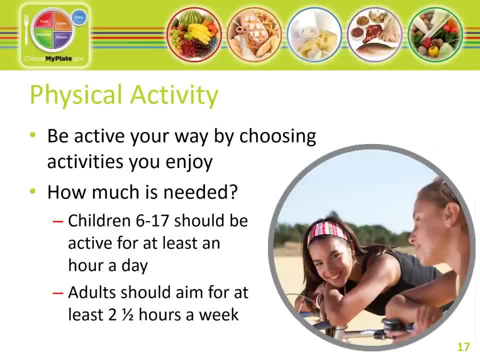 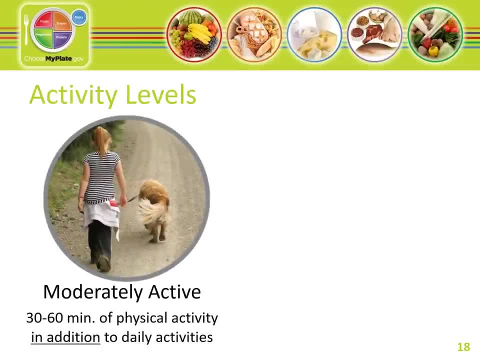 will stay in line, you have more energy and, chances are, you'll feel happier. You can choose moderate or vigorous activities, or a mix of both each week. The level of intensity is based on the extent to which the activity makes you breathe harder. 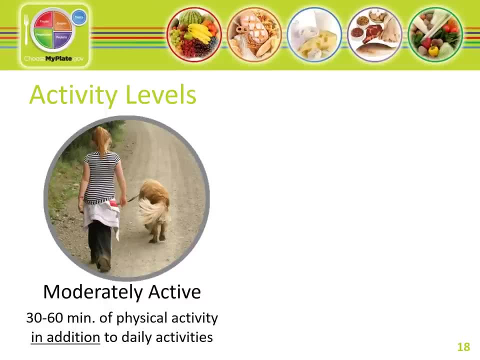 and your heart beat faster. Only moderate and vigorous intensity activities count towards the highest level of intensity. The level of intensity is based on the extent to which the activity makes you breathe harder and your heart beat faster. The level of intensity is based on the extent to which the activity makes you feel faster. 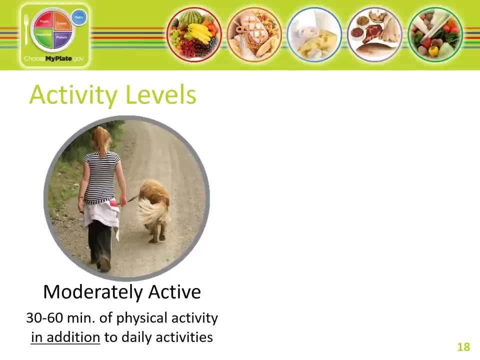 and your heart beat faster. The level of intensity is based on the extent to which the activity makes you feel faster and your heart beat faster. Try to limit sedentary activities like sitting for a long period of time, watching TV or using the computer. 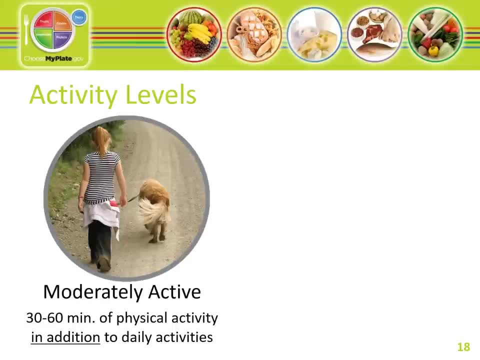 With vigorous or active activities you get similar health benefits in half the time it takes you with moderate ones. You can replace some or all of your moderate activity with vigorous activity. Although you are moving, light intensity activities do not increase your heart rate. 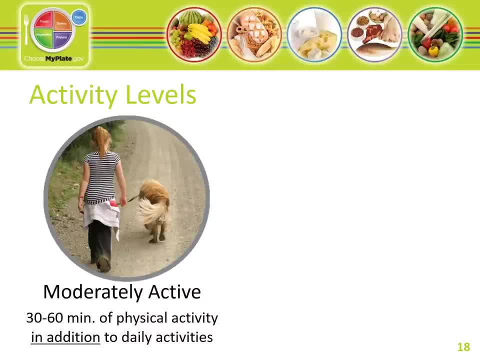 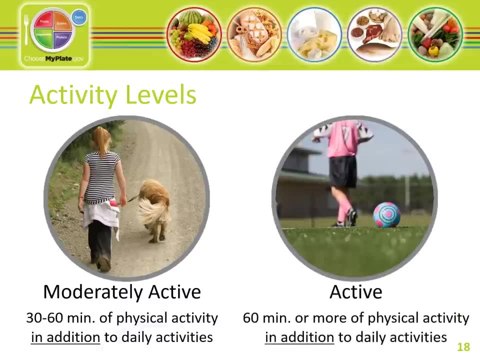 You should not count these towards meeting the physical activity recommendations. These activities include walking at a casual pace, shopping and doing light household chores. If you're not being very active now, increasing your strenuous activities will make you feel better and tone your body. 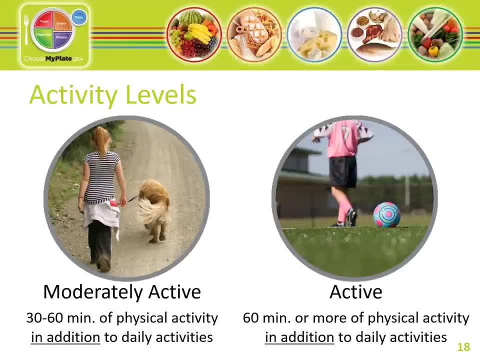 Some examples of moderate activities include: walking at approximately 3 mph. general gardening like raking, trimming shrubs, dancing water, aerobics, canoeing and tennis. Examples of vigorous or active physical activities include running or jogging at approximately 5 mph. walking very fast at about 4.5 mph. bicycling, more than 10 mph. heavy yard work. 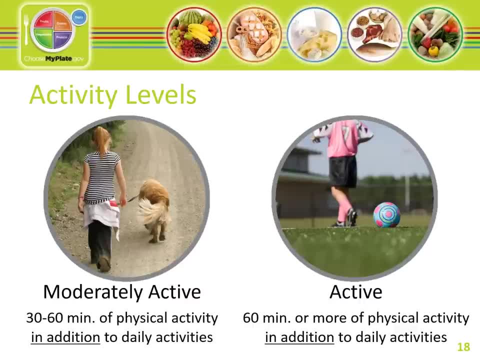 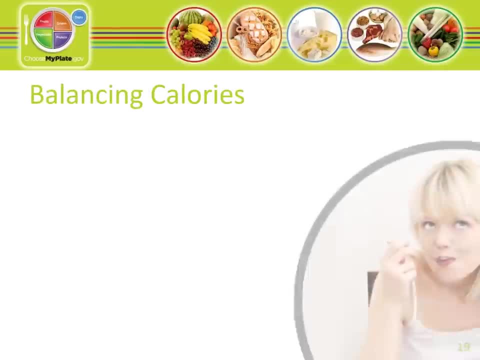 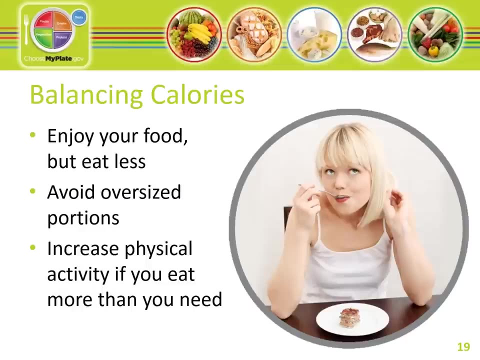 such as chopping wood, swimming, aerobics and swimming. A main message of MyPlate is calorie balance. Calorie balance refers to the relationship between the calories you get from the foods you eat and drink and the calories you use by being active. 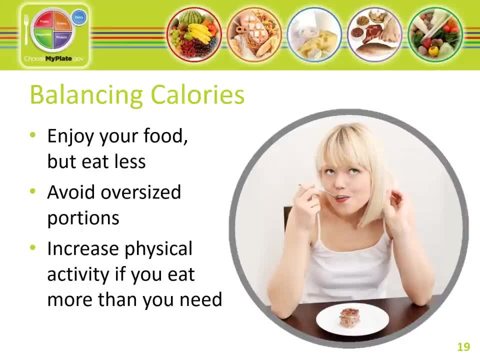 If you want to know the number of calories you should eat in a day, you can get your personal daily calorie plan at wwwchoosemyplategov. Thank you for watching. I'll see you next time. Bye. People who are successful at managing their weight have found ways to keep track of how. 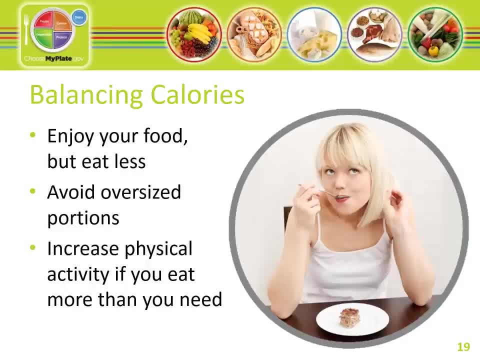 much they eat in a day, even if they don't count every single calorie. Tips for balancing calories include avoiding oversized portions. Piling your plate or having too much food on your plate leads to oversized portions. Use a smaller plate, bowl and glass. 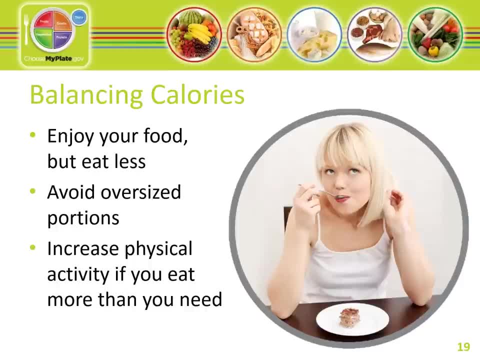 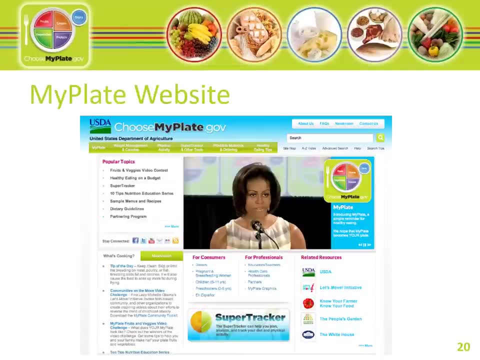 Stop eating when you feel satisfied, not full. Take your time to eat. Enjoy your food. The MyPlate website has numerous tips, suggestions and interactive activities to help you eat well. Take time to check out this valuable resource. Can you visualize what your plate would look like today? 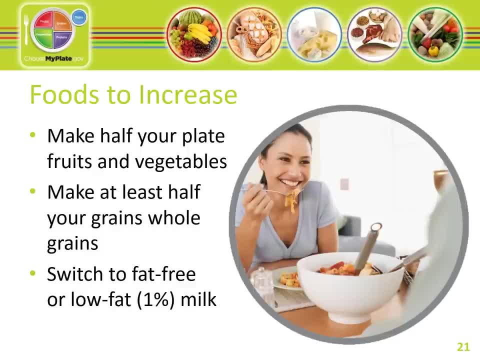 Are there foods you need to increase? Maybe you're eating too few vegetables, fruits and vegetables. Keep that in mind as you eat, Or you can also use your food for your diet. You can also eat foods that are high in calories. 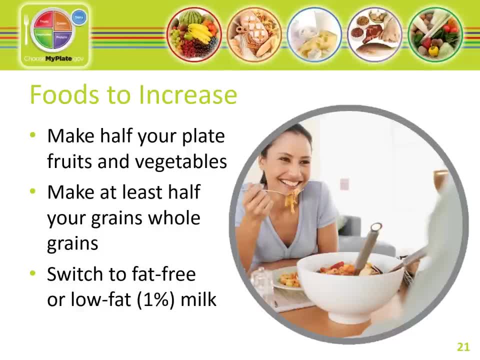 That's what I will talk about today. I hope you enjoyed this video. fruits, whole grains or dairy products. Keep in mind that in order for you to get all your essential nutrients and remain healthy, you need to make healthful eating a habit. 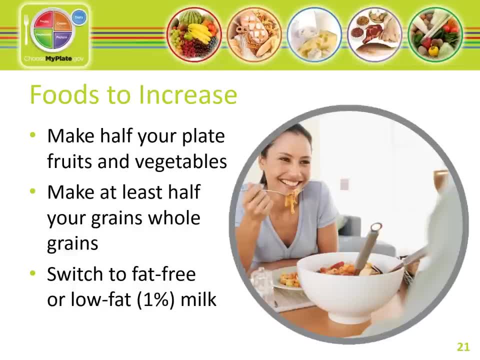 The good news is, if you move to the MyPlate model and if you choose lots of different foods and food groups, those missing nutrients will be found. Remember these tips for the foods you should increase: Make half your plate fruits and vegetables. Make at least half your grains- whole grains. 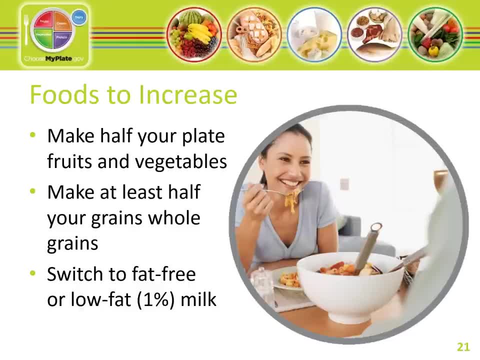 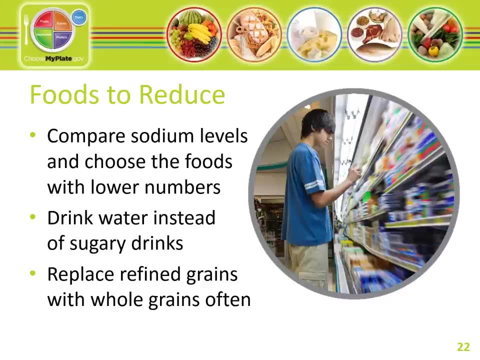 And switch to fat-free or low-fat, 1% milk. Certain foods and food components, if eaten in excess, can increase your risk for health problems later in life. These include sodium or salt, saturated fat, trans fat, added sugars and refined grains. 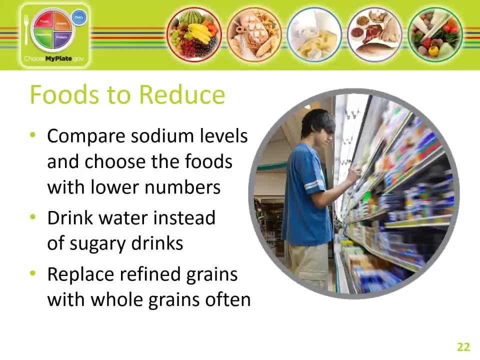 Knowing what is in food comes from reading labels and requesting nutrition information for your diet. When eating out at restaurants, cut back on foods that contain a lot of empty calories and foods that have been overly processed. When you fill up on too many of these foods, you don't have an appetite for healthy foods. 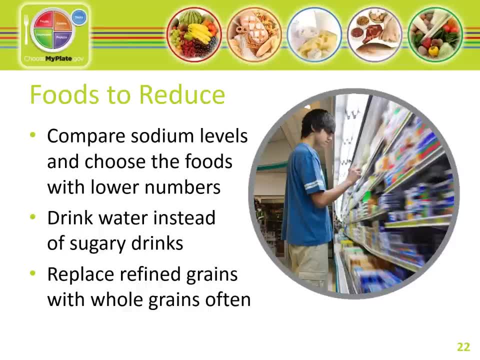 Remember these tips for foods to reduce. Compare sodium levels in soup, bread and frozen meals and choose the foods with the lower numbers. Select canned foods labeled low sodium, low sodium and low sodium. Reduce sodium or no salt. added Drink water instead of sugary drinks. 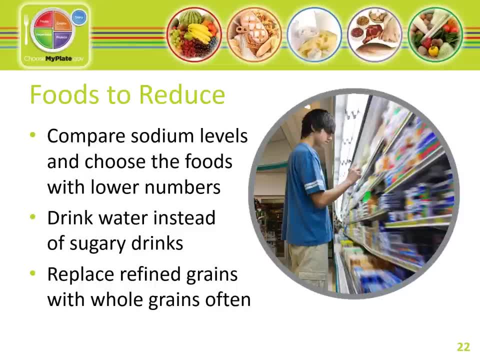 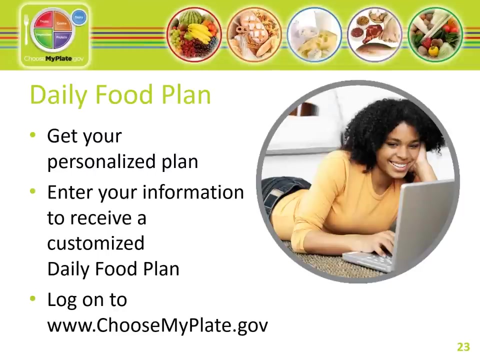 Remember that soda, energy drinks and sport drinks are a major source of added sugar and calories in American diets. Replace refined grains with whole grains. often Try eating whole wheat bread instead of white bread or brown rice instead of white rice. If you want to know the amount of each food group you need daily, you can use MyPlate for 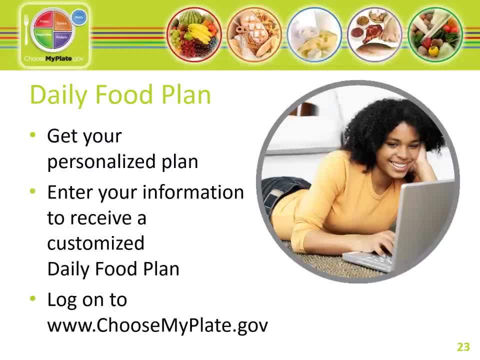 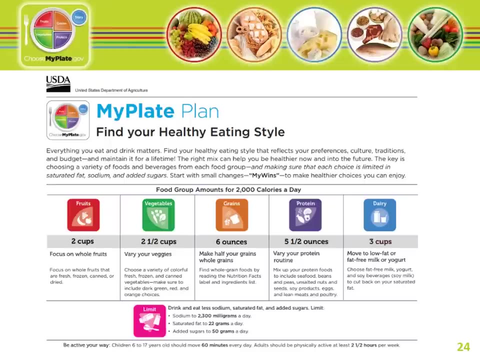 the quick and easy decisions of what to eat. You can get more detailed information on the MyPlate website, wwwchoosemyplategov. Enter your information to receive a customized daily food plan. The MyPlate plan lets you know how much food you should be eating from each food group. 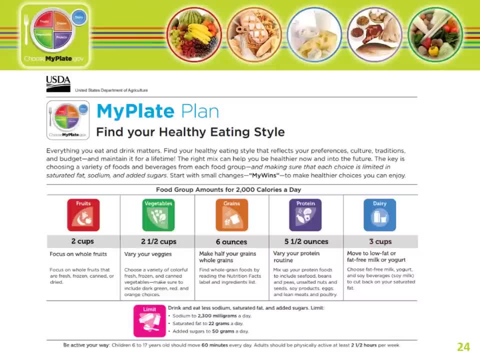 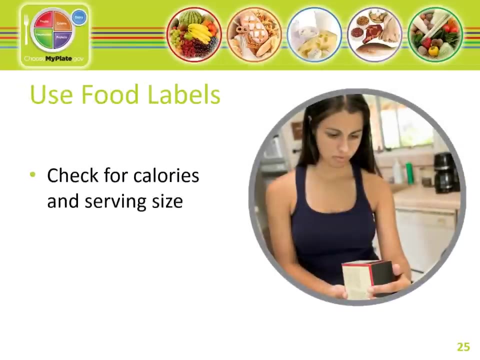 daily. The MyPlate plan lets you know how much food you should be eating from each food group daily. You can read nutrition tables to learn the konkret様's options in bothhaps. The MyPlate plan lets you know how much nutrition you should be eating from each food group. 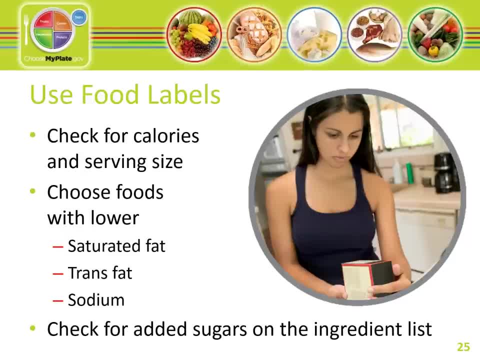 daily. Anyone who eats too much can be found on the MyPlate website, which is one of the honest ould options, or on Facebook, where you can make personalite choices. little time to get used to what to look for, but once you find where to look, it makes identifying. 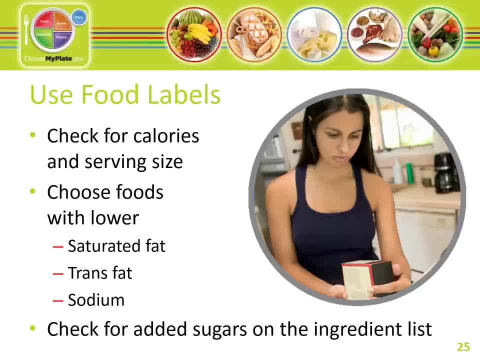 good food choices easier. Check for calories on the nutrition facts panel. Compare that number to your calorie level from your daily food plan. Look at the serving size and compare that with how many you will eat or drink. If you double the serving you eat or drink, you double the calories. 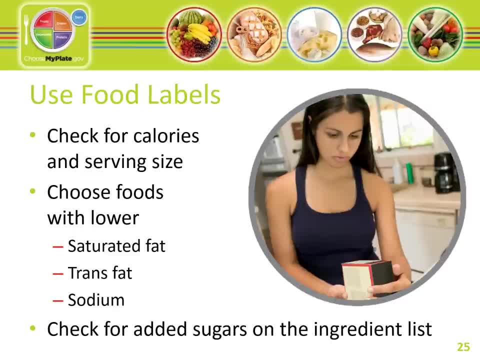 Look at other brands or types of the same food. Choose foods with lower calories, saturated fat, trans fat and sodium. the difference can be big. Check for added sugars using the ingredient list. Some names for added sugars include sucrose, glucose, high fructose, corn syrup, corn syrup. 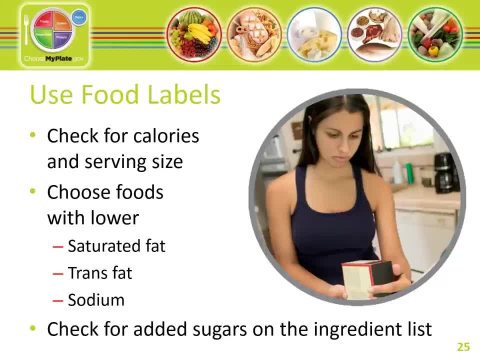 maple syrup and fructose. If the food is a grain food, such as cereal, crackers or half fat food. check for added sugars. Add added sugar if you don't have sugar or pasta. is the first ingredient a whole grain. Choose whole grain foods over.